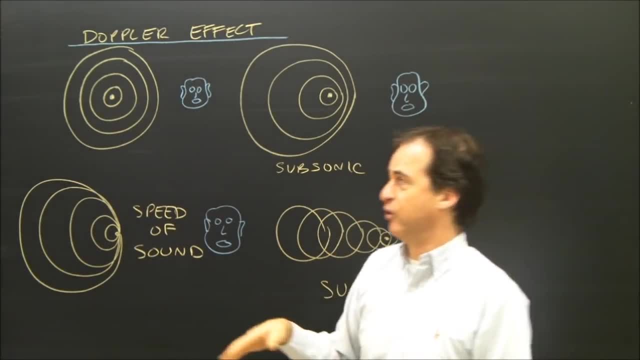 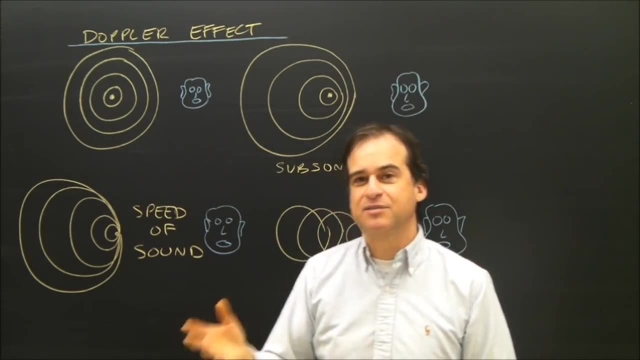 A frequency of like 220 hertz would be a lower note. So these waves, this person hears these sound waves as they pass by their ear If the object that's making the sound is moving, and let's say it's moving at subsonic speed, which means it's moving less than the speed of sound. 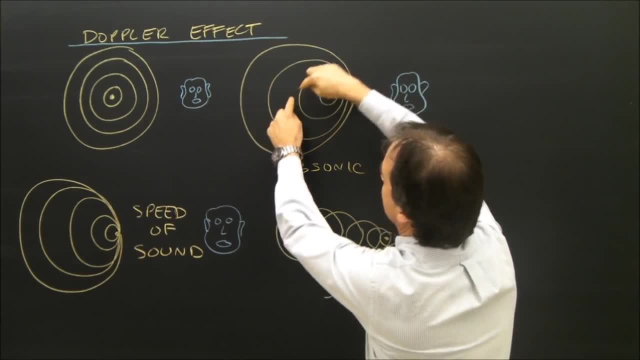 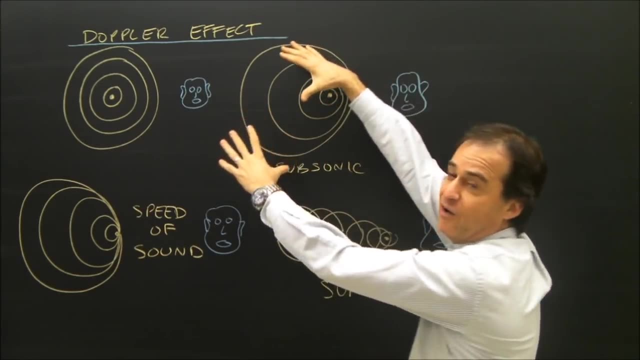 then the first wave here was made when the object was over here. The object is moving this way: When it was here, it made this sound wave And that sound wave radiates out. And when the object's over here, that sound wave had already gotten to be this big and it's still radiating out. 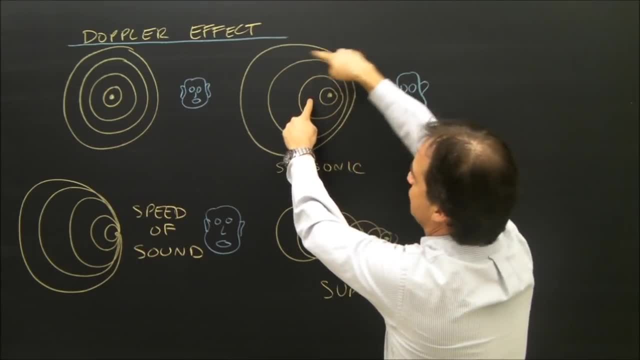 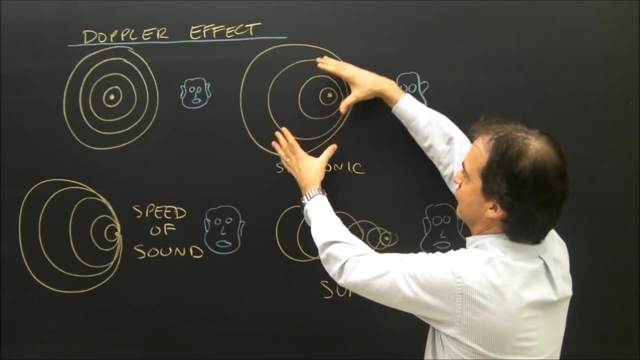 This sound was created when the object was here, and that's why it's around that point. This sound wave was created when the object was here. So the object creates a sound wave, then moves, creates another sound wave, moves, creates another sound wave. So, as the sound is leaving the siren, the sound waves on this side are starting to bunch up, which means this person hears more of these waves pass in a second than they heard when they were over here. Even though these sound waves are traveling the same speed, once the siren sounds leave, they travel the same speed in air. 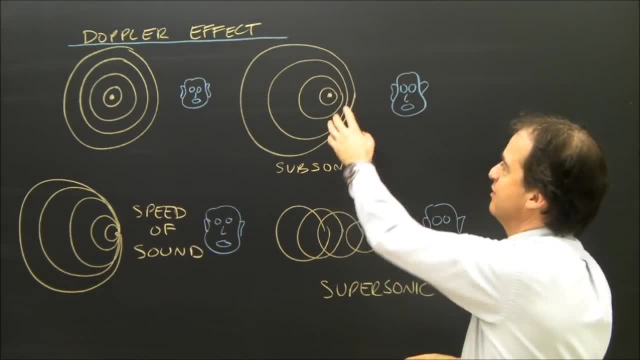 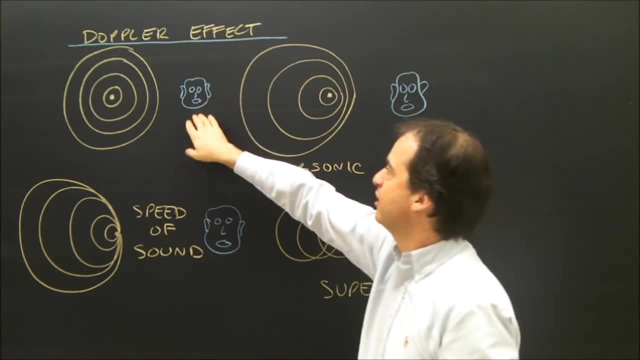 But because the object is moving, these sound waves are getting bunched up And so this person hears a higher-pitched sound going by them. But this person over here listening to this object, the sound waves getting to him. well, they're spread apart further. 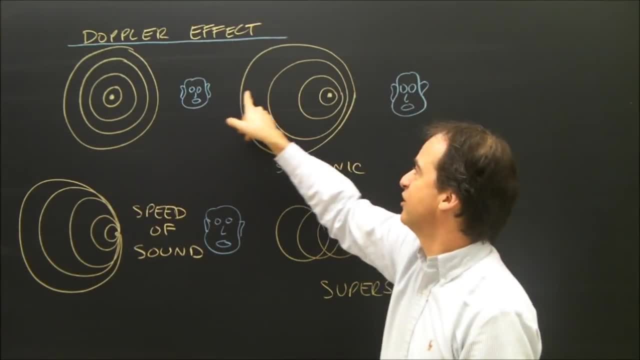 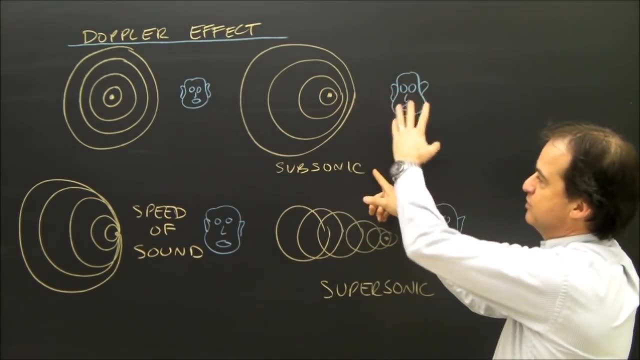 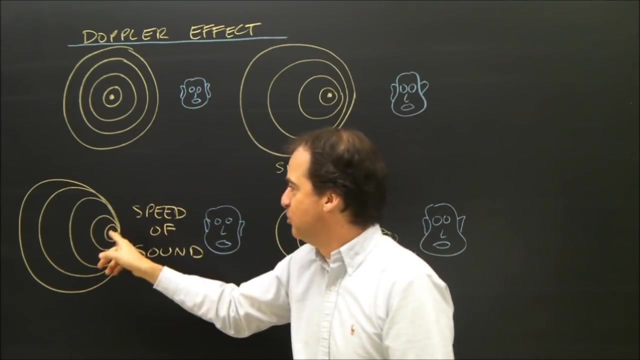 So their frequency is lower. This person hears these sound waves as a lower note. So if you're standing here as the sound goes by, it gets higher-pitched one frequency and then lower-pitched frequency. Now, if the object actually travels the speed of sound, then as it's moving, it created this circular wave when it was over here. 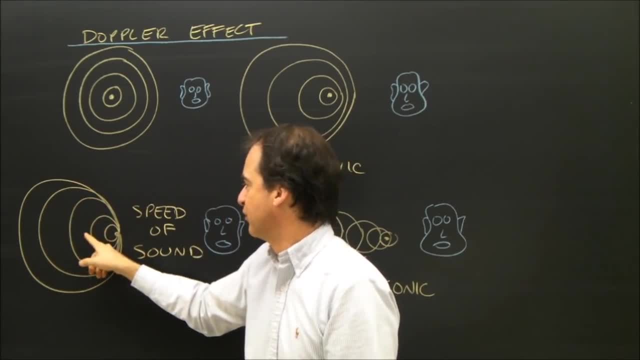 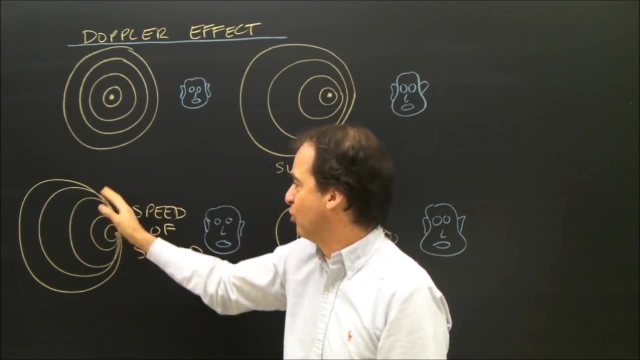 And then it created this circular wave when it was over here. At this point it's over here creating another circular wave, And if you look, all the crests of these waves are bunched together all in the same line. It's as if all that sound energy, all the energy of the sound, 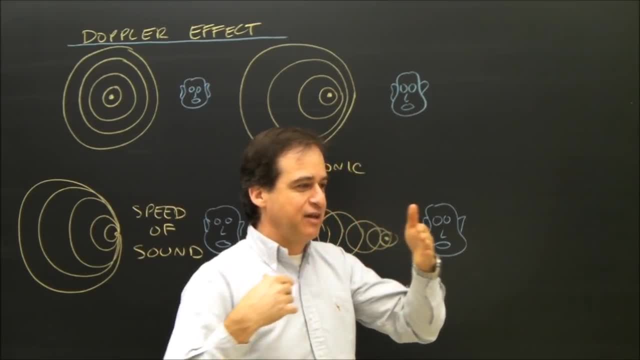 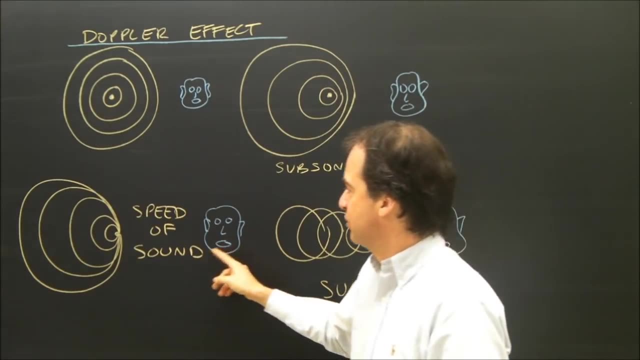 is bunched up there. I make a sound wave and as it's leaving me, I'm running at the same speed as that sound wave and I'm making another sound wave. They're all bunched up here, So this person would hear sort of a loud noise as this went by. Because they're hearing all that sound all at once, And so it's a lot of pressure in that wave and you'd hear a slightly like a boom. If the object is traveling faster than the speed of sound, we have a similar thing happening. 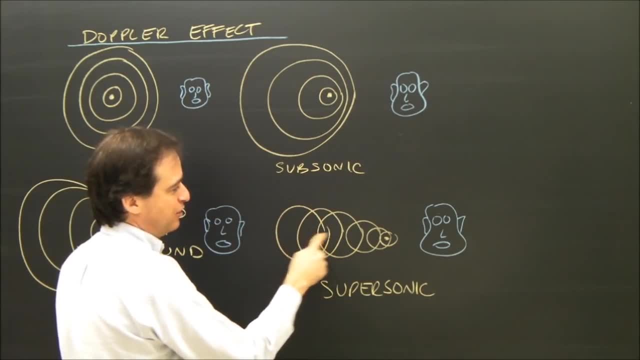 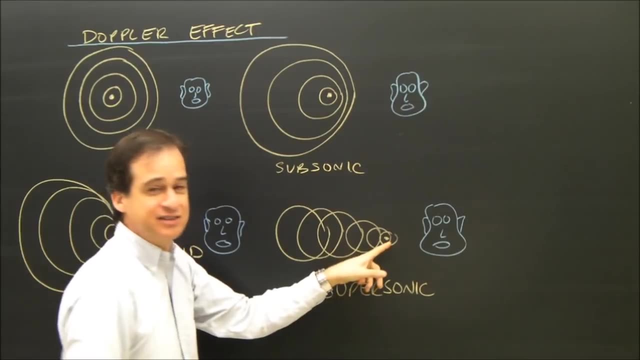 Except this sound wave was made when the object was moving. This sound wave was made when the object was here. This one was made when the object was here. The object's all the way over here And this sound wave is not radiating out as fast as this thing is moving.